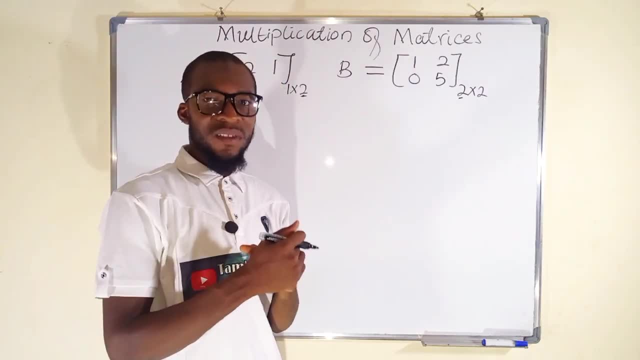 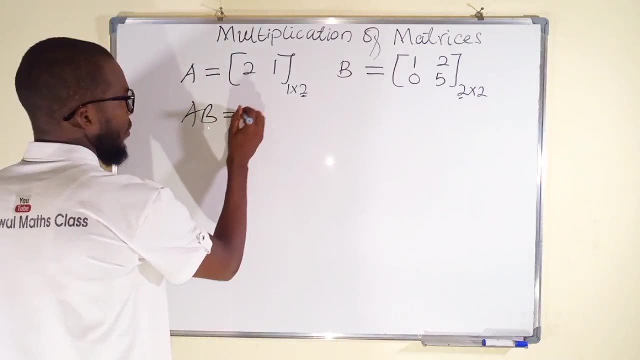 to two. the number of columns here and the rows here must be exactly the same before you carry out this multiplication. all right, one important thing is that we have to consider the columns here and the rows- and the rows here must be exactly the same- before you carry out this multiplication. all right? 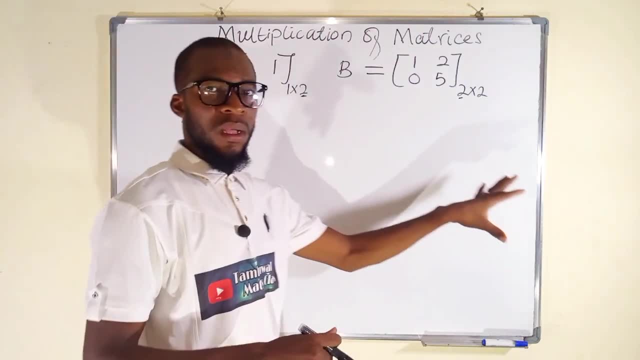 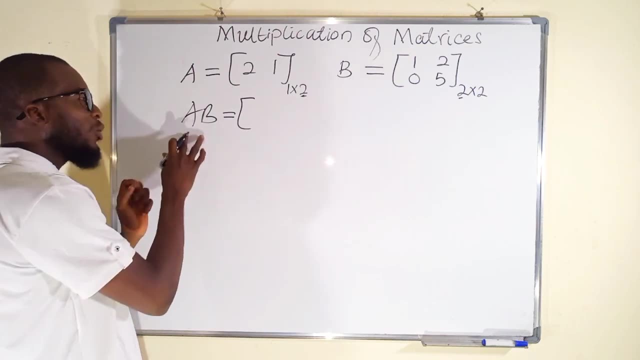 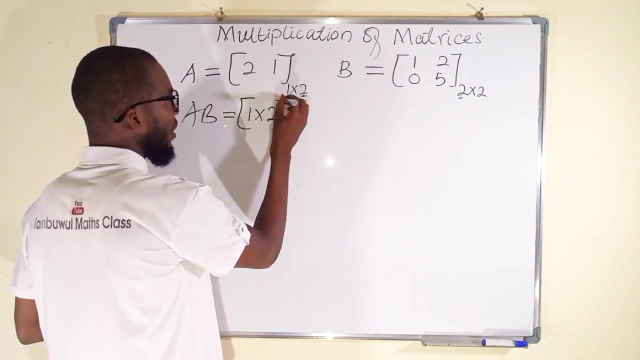 one important thing is that we have to consider the columns here and the rows here must be exactly the same of this order is that it determined the order of the result after multiplication. so, after multiplying matrix a and b, the order of the result will be one by two matrix, we are going to obtain a matrix of. 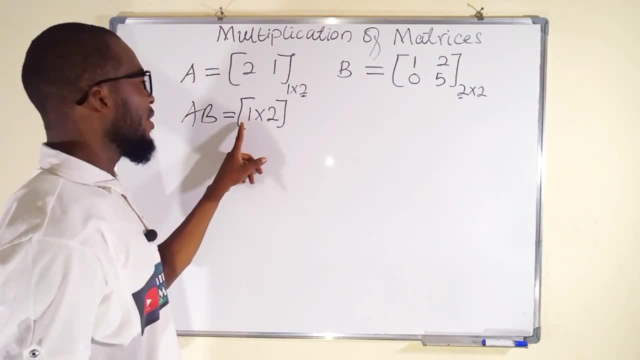 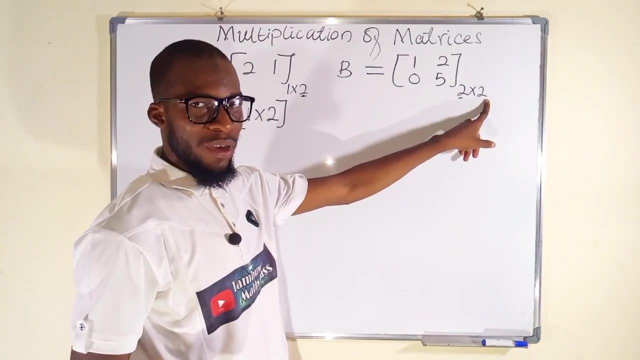 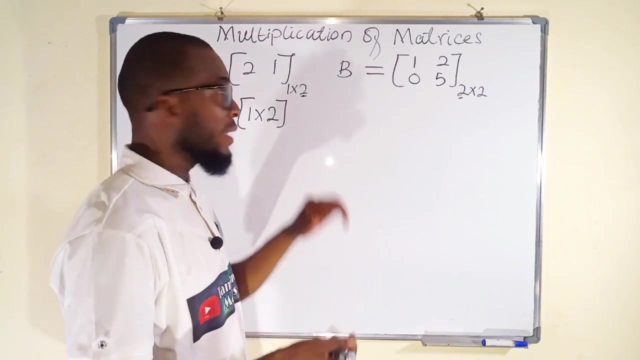 dimension one by two. one here stands for the number of rows from the first matrix, and two here is the number of columns from the first matrix, and two here is the number of columns from the circle matrix. So you see, this order has two advantages here. One: it can help to determine. 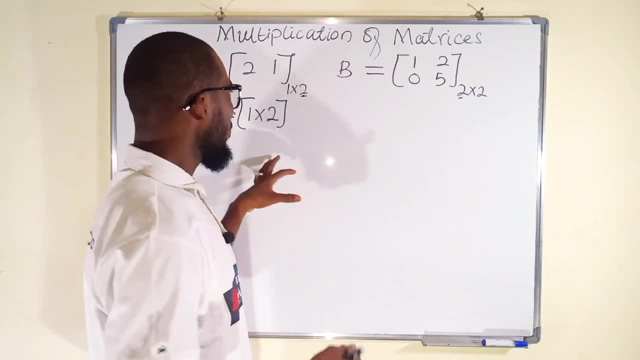 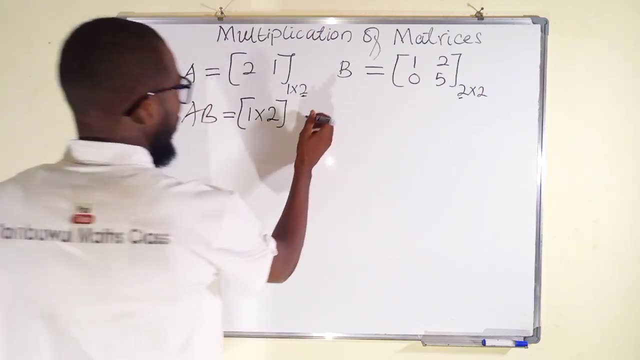 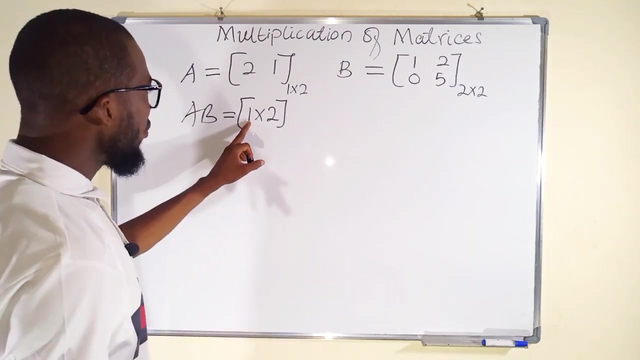 whether the matrix can be multiplied And, secondly, it can determine the order of the result after multiplication. Okay, so now the question is: how can we multiply these two matrices together, Since we know we are going to obtain a single row and two columns after multiplication? 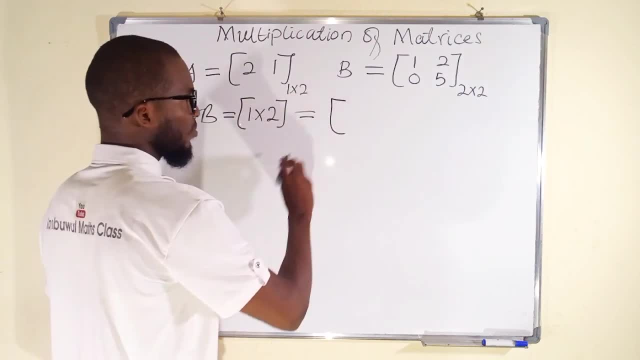 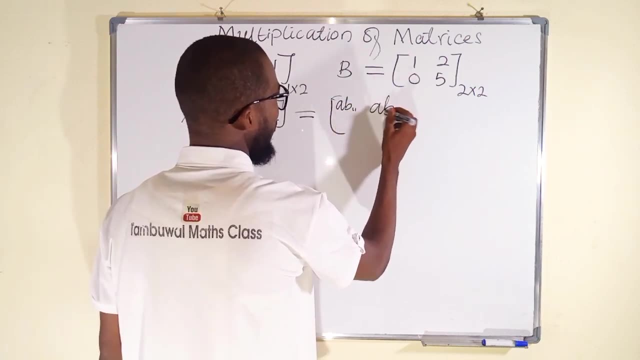 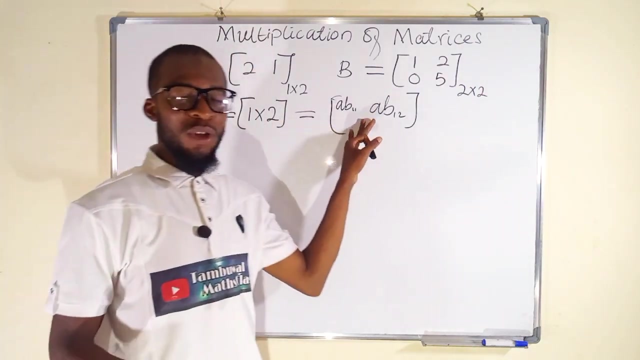 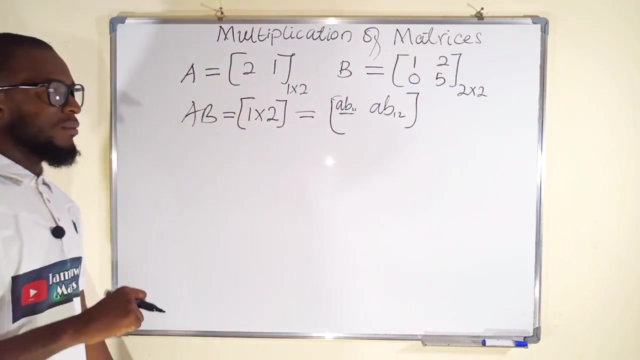 So it is going to be of the form. let me call it AB11, AB12.. This is going to be the form of the matrix. we are going to obtain Two columns, Two columns To obtain this term here, this element. we are going to multiply the whole of this row. 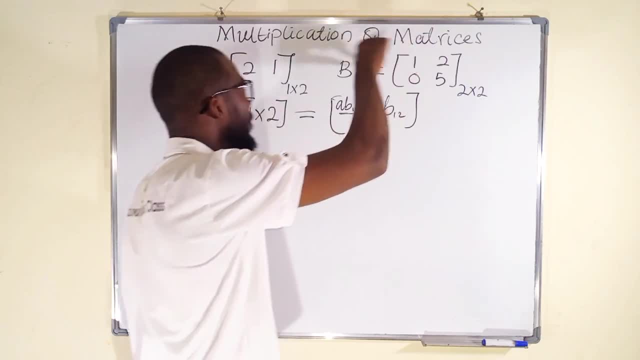 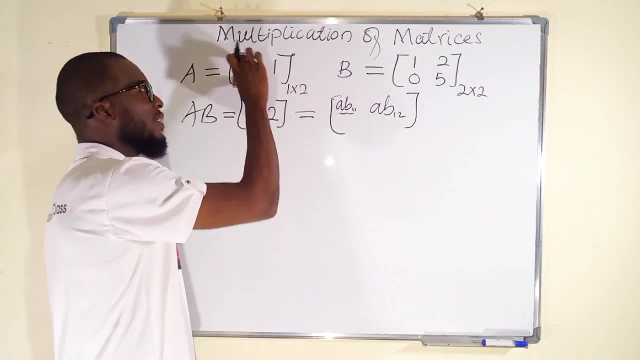 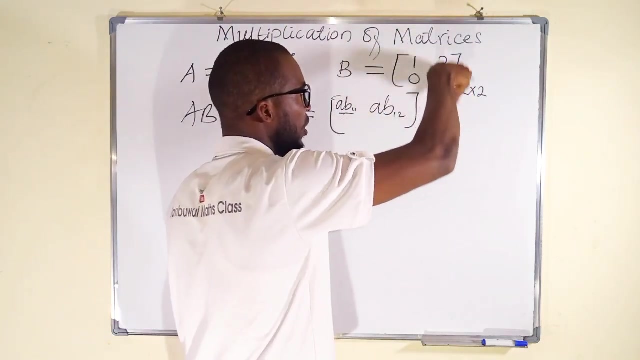 by the whole of this column, That is, first row, first column, to obtain this one. And for this we take the first row. already we already have a single row. we take the row and multiply by the second column to obtain AB12.. 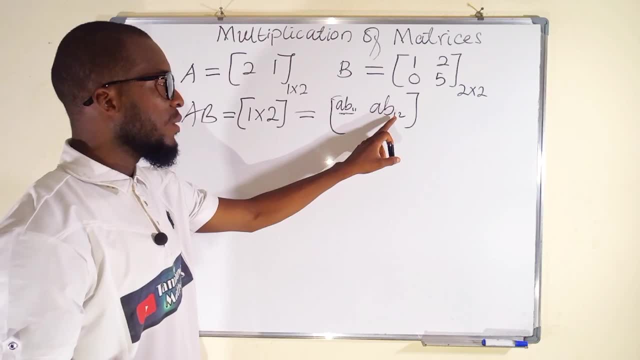 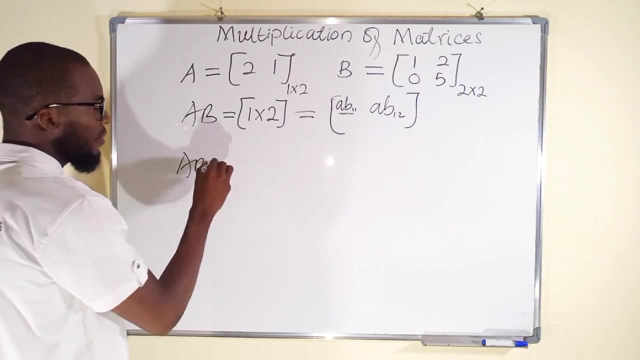 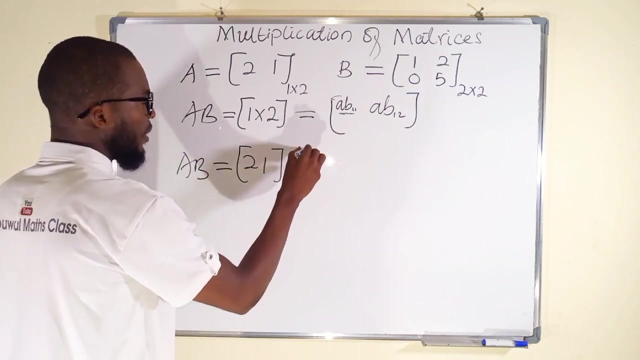 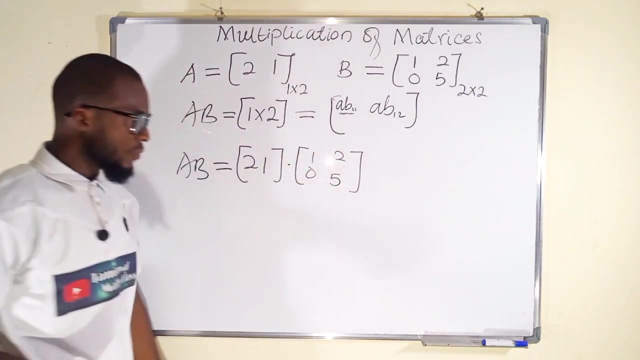 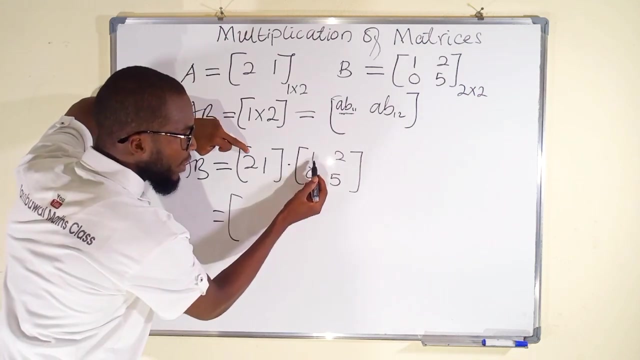 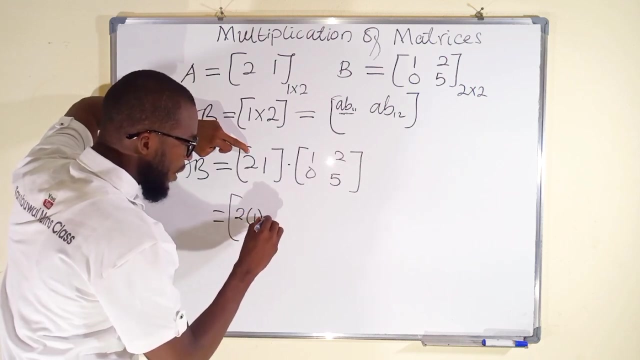 That is an element in the first row, second column. So let us begin. AB will be equal to 21 multiplied by 1025.. This is equal to: we take the first element here, we multiply by the first element. here we have 2 multiplied by 1, then we add. 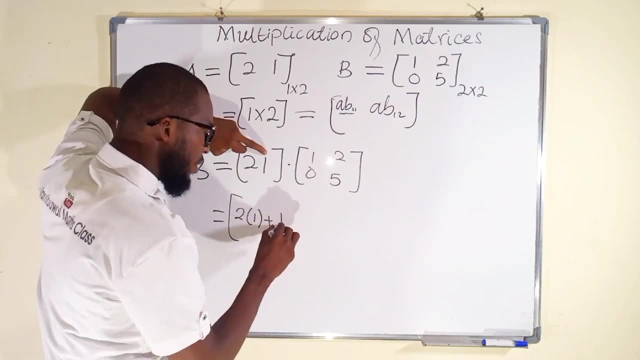 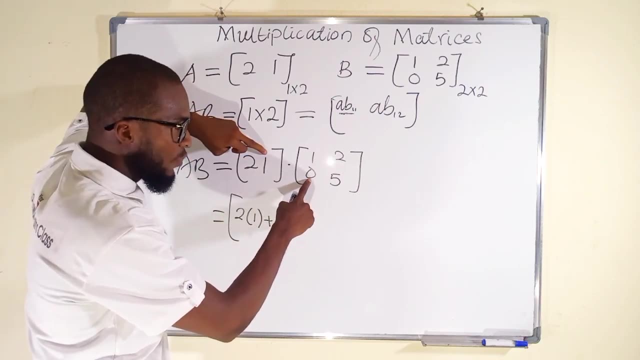 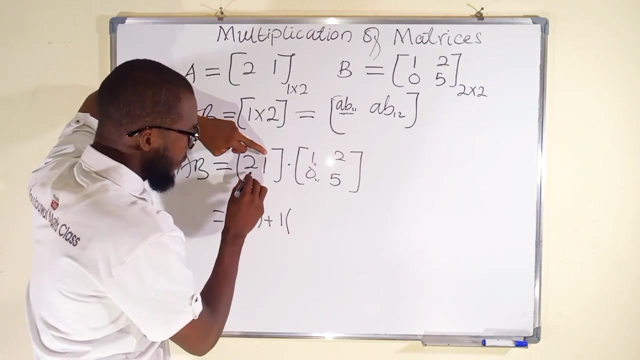 We take the second element here, which is 1, we multiply by the second element here at 2, 1.. 2, 1 position. This is 2, 1 position. This is 1, 1 position. 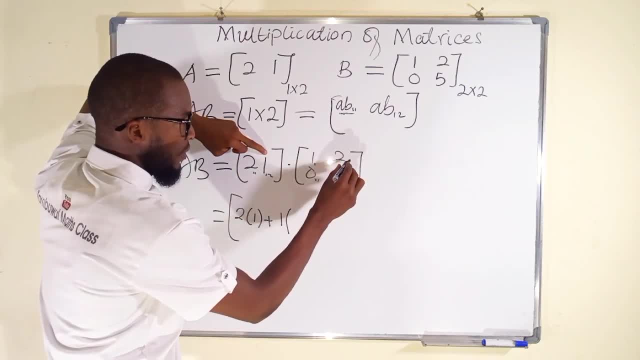 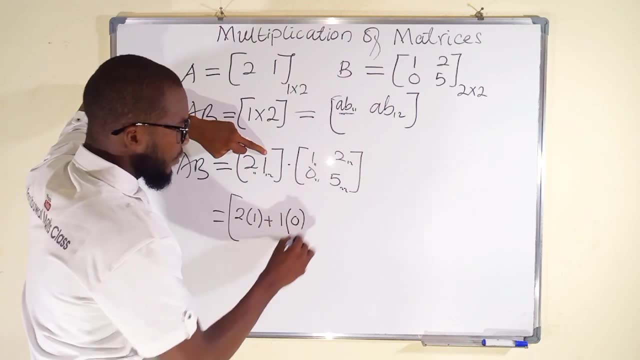 This is 1, 1 and 1.. This is 1, 2.. This is 1, 2.. This is 2, 2.. We take this, we multiply by this, We are done with AB11.. 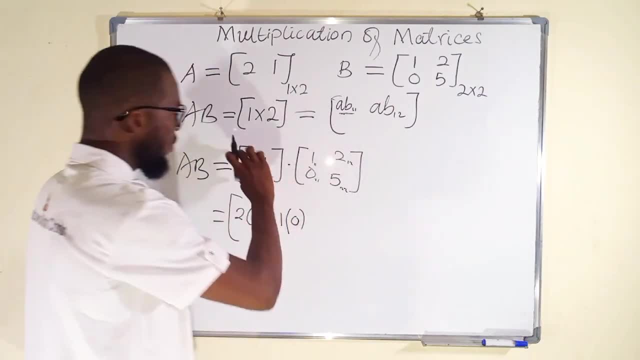 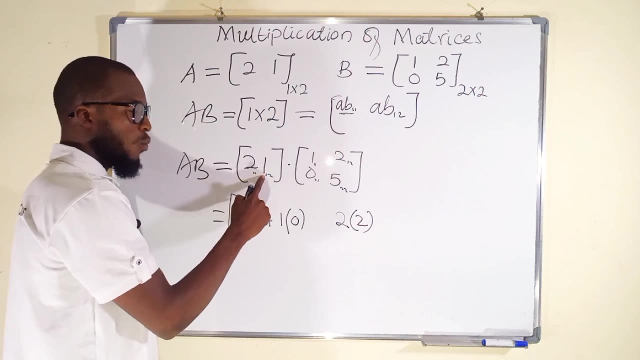 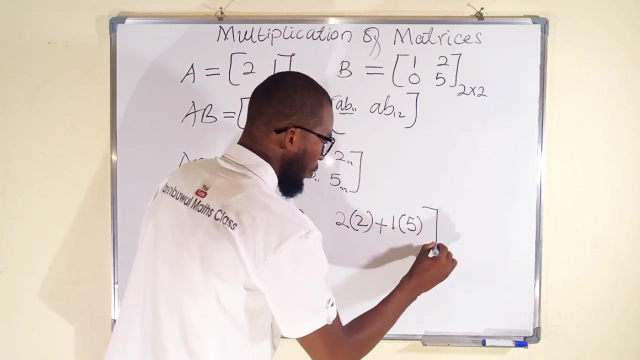 We give it space because we only have two elements. We take this one again: 2 multiplied by this 2, 2 multiplied by 2, plus 1 multiplied by 5.. we close and simplify to obtain our final answer. you know, this time this is. 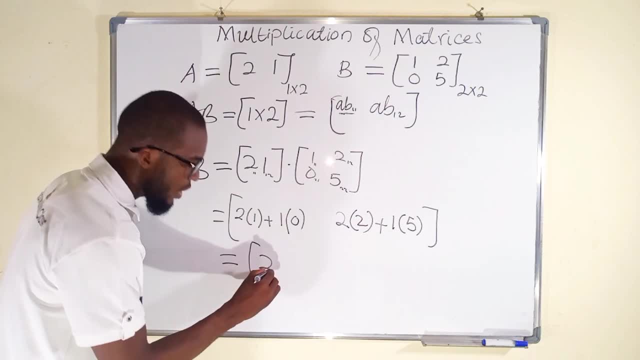 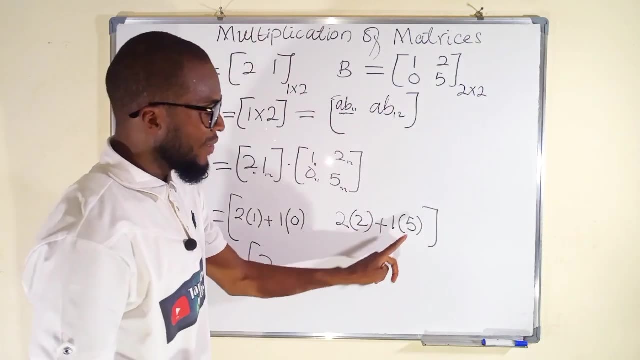 0. this time this is 2, so we only have 2 here. they will move to the next line we have: 2 times 3 is 4, then 1 times 5 is 5, so we have 4 plus 5 is 9. we have 9 here. 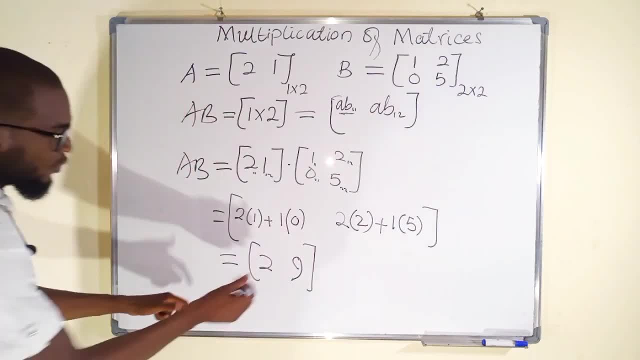 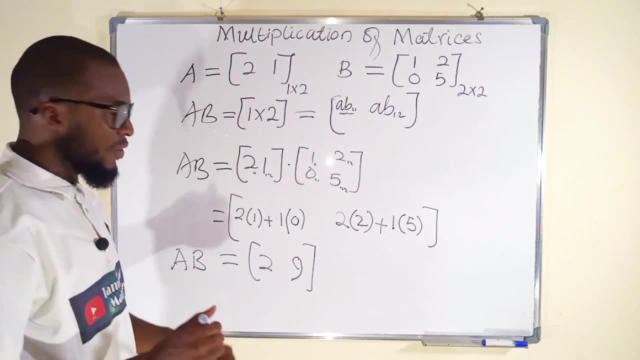 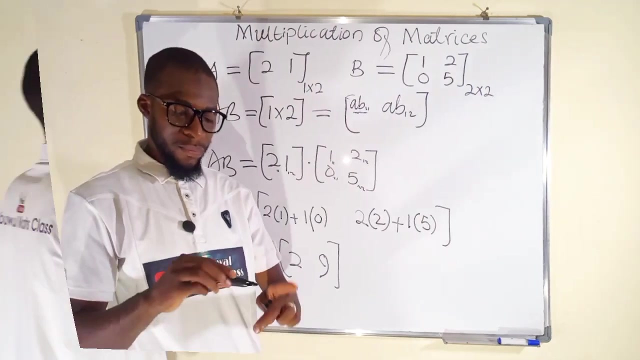 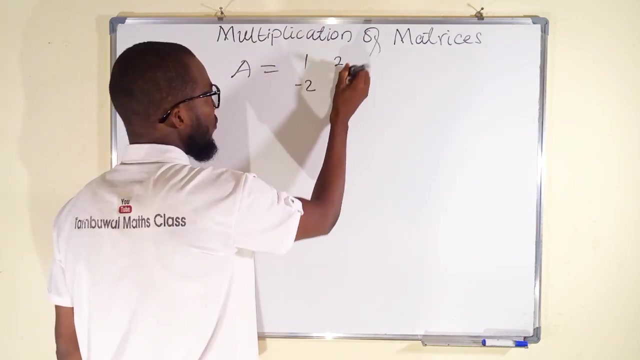 so you can see that the only two elements we have are 2 and 9, which is the result after multiplying A and B together. so this is how to multiply matrices. let us take further examples. so first we have a matrix, A as 1 minus 2- 2. 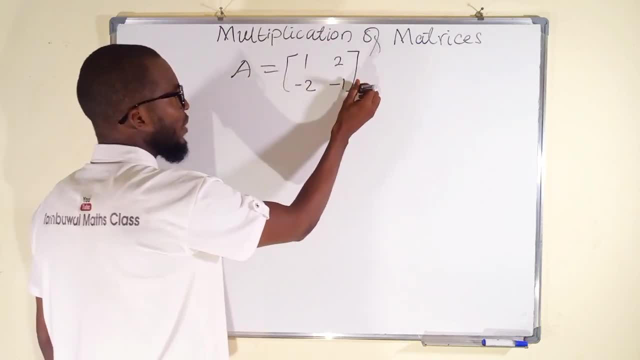 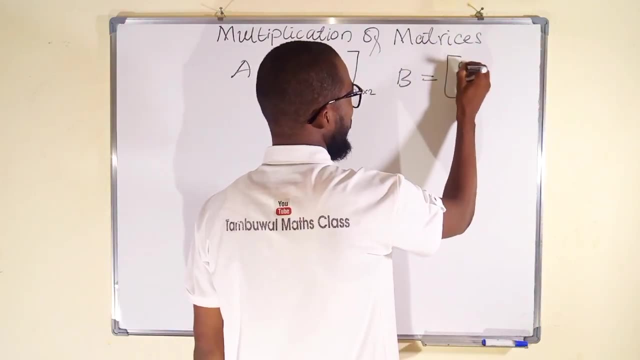 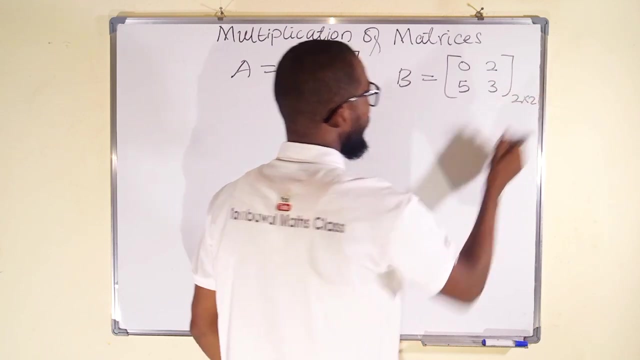 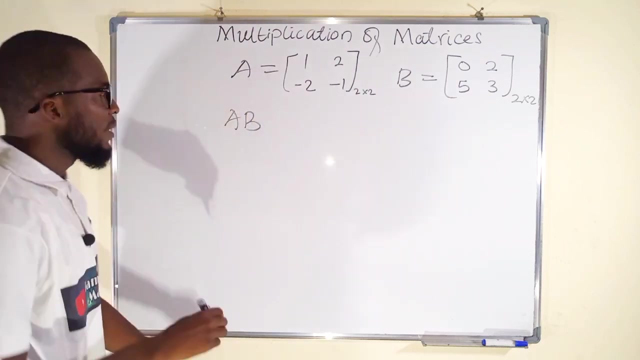 and minus 1. this is a matrix of 2 by 2. and we have another matrix B of the same dimension, maybe 0, 2, 5 and 3 is also 2 by 2. we want to multiply A and B together. first thing to. 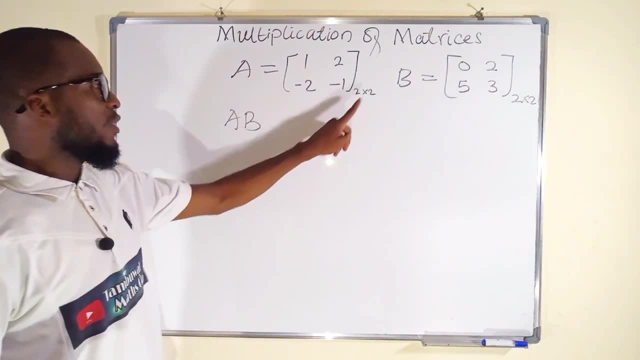 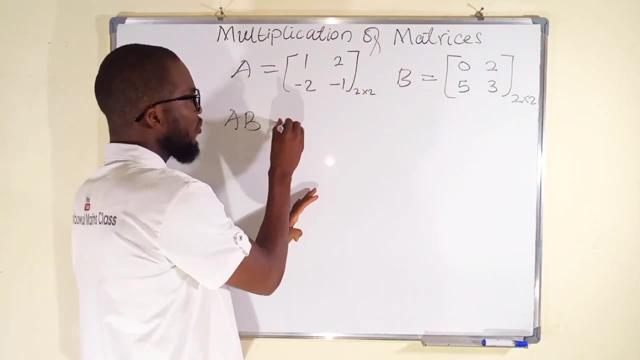 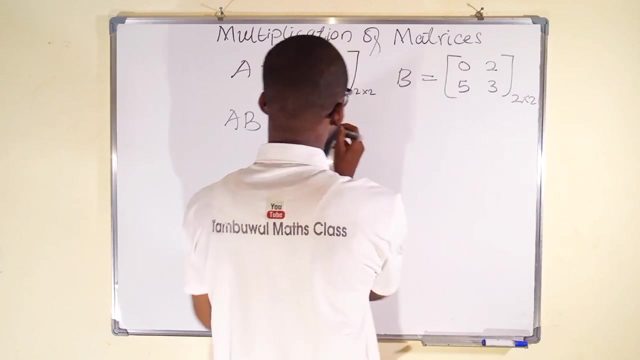 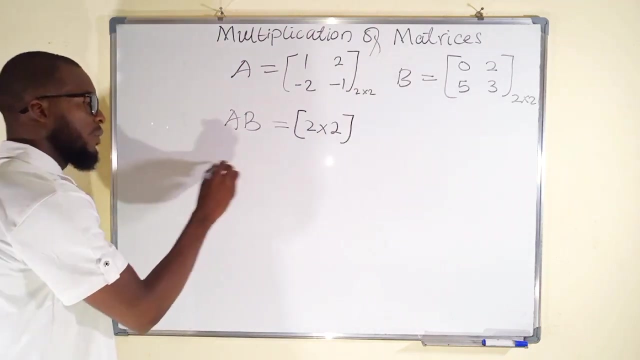 check is for the compatibility and the number of columns here and the number of rows here. you can see they're exactly the same and for the result it is going to be of a dimension. you check for the number of rows here, which is 2, number of columns here too. so we are going to obtain a matrix of 2 by 2. so let's start. 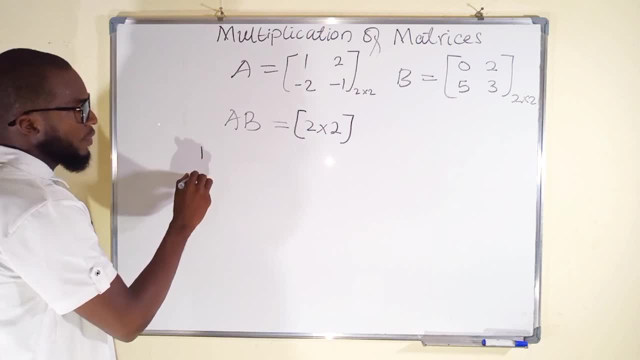 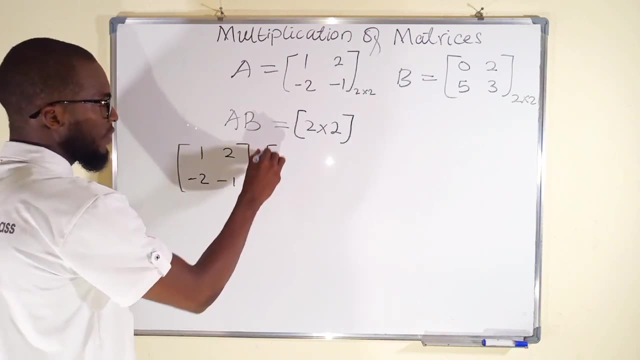 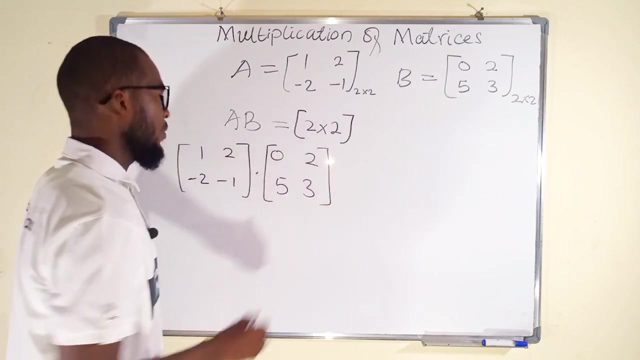 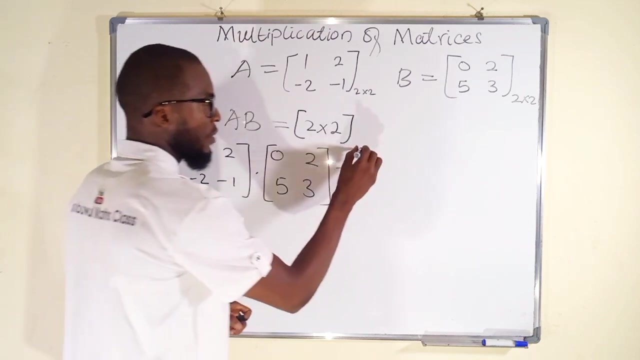 we have a matrix A as 1 minus 2, 2 minus 1. we want to multiply that with that other matrix. okay, this is going to be, I told you, because it is two by two. um, this is how it's partially going to be to obtain the first element. 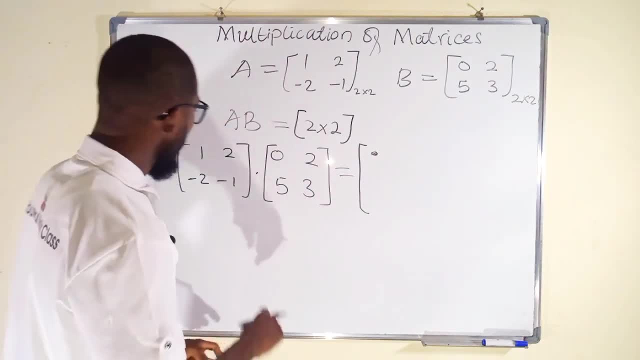 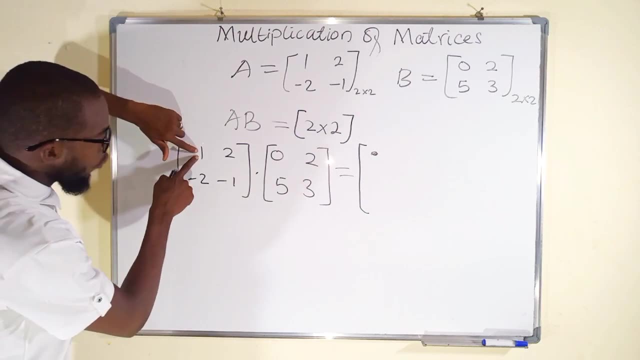 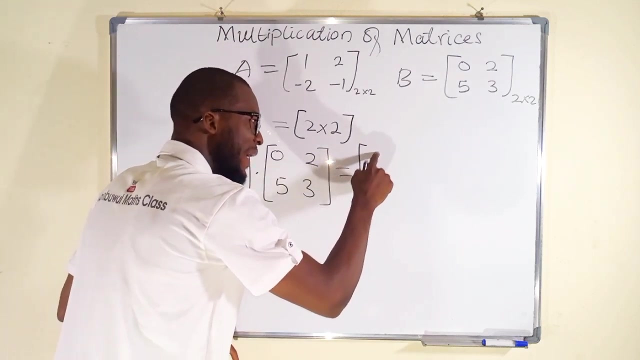 here at one one's position. we're going to take the first row here and multiply with the first column. here we take one multiplied by zero, we add, we take two multiplied by five to obtain, uh, an element here at one one's position. so let's do that. we have one multiplied by zero. 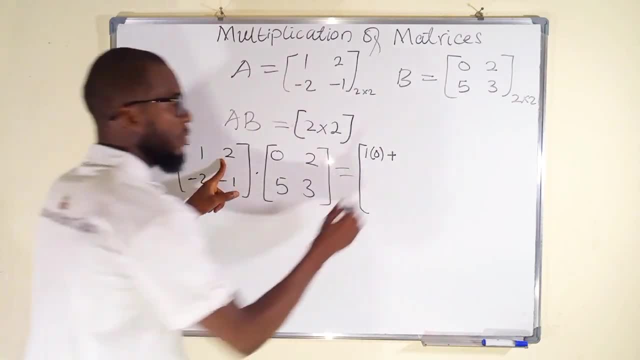 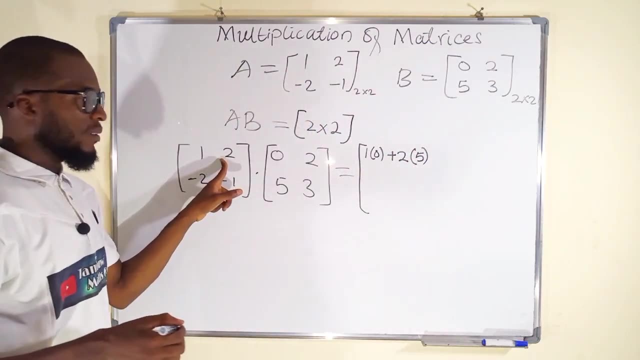 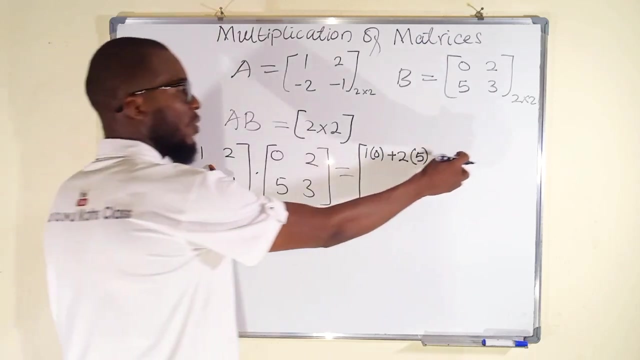 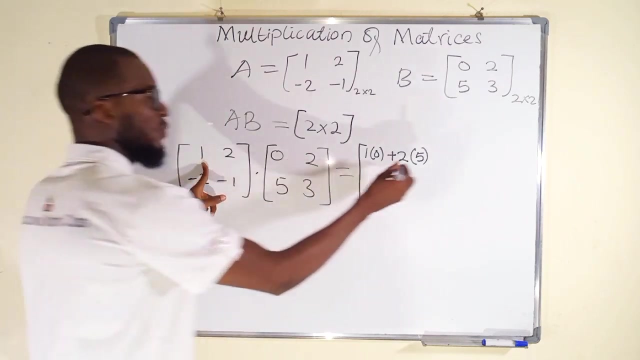 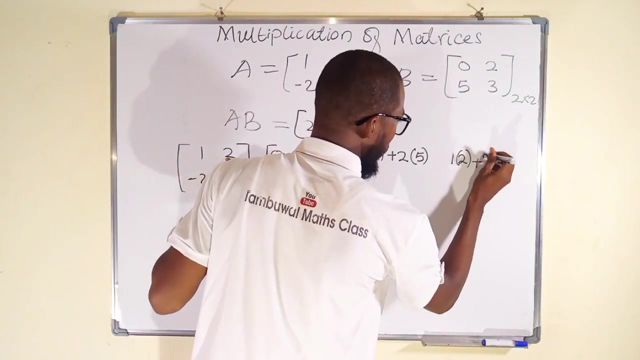 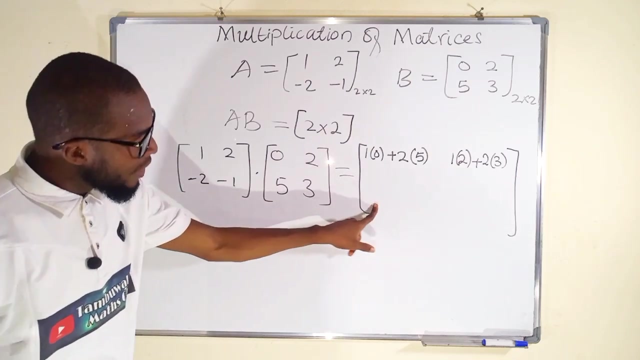 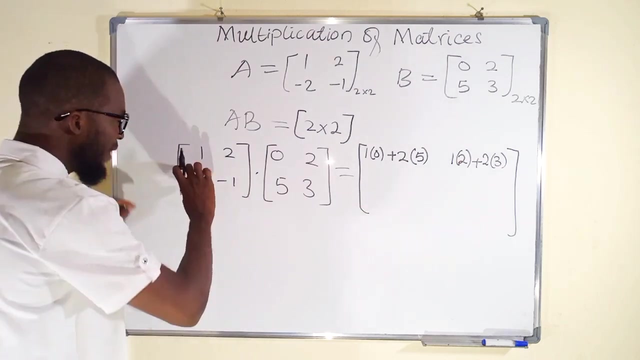 then we add, we take two, we multiply it by five, we are done with this. then we give a space, we take the same row multiplied by the second column to obtain, uh, one tooth position. so one times two plus two times three, and we are done here. then, to obtain this element, here at two, one position, we take the second row multiplied by. 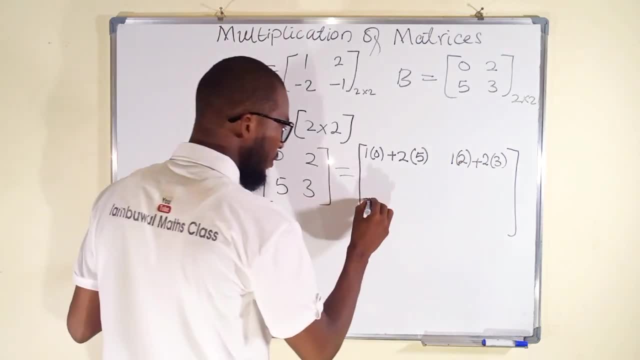 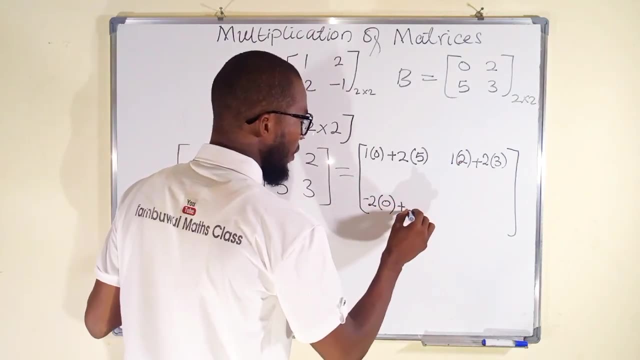 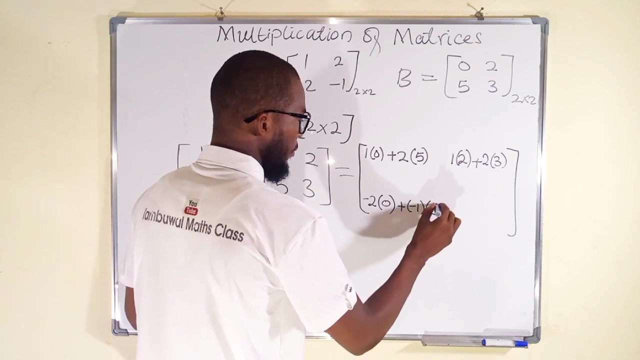 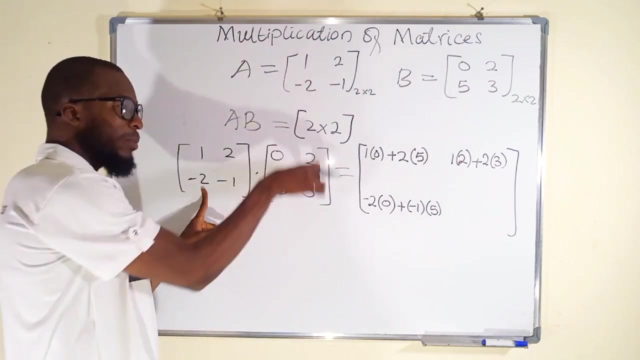 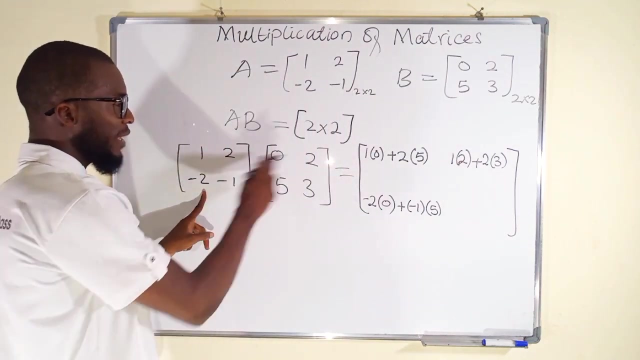 the first column. we have negative two multiplied by zero, plus we have negative one multiplied by five. we give a space. we take the same row, second row, multiply by the second column to obtain the two. two position element. we have negative one times two. okay, it is negative two. 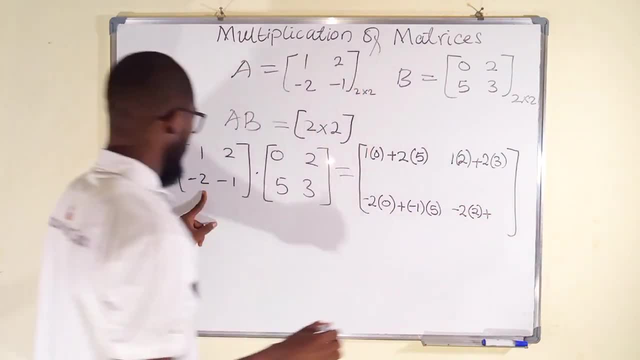 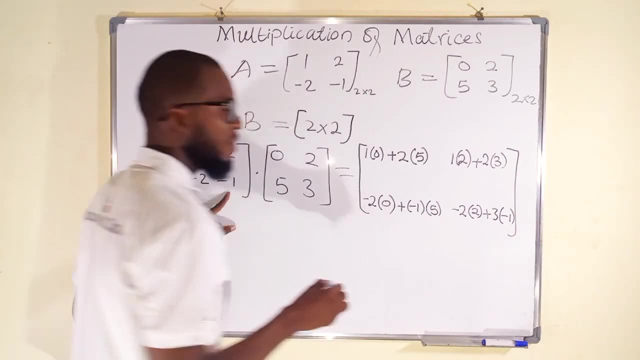 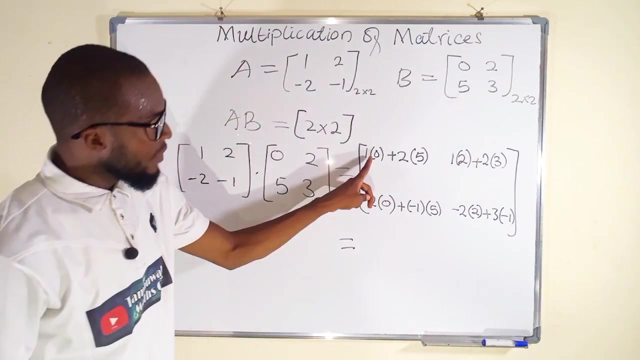 and times two we add, then we take negative one times three, we can write it as three times negative one, all the same commutative. all right, now let us simplify and obtain our final answer. this is zero, this is ten. ten plus zero is ten, so we have ten here. 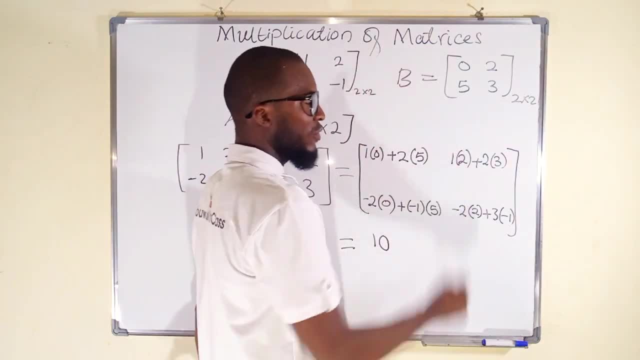 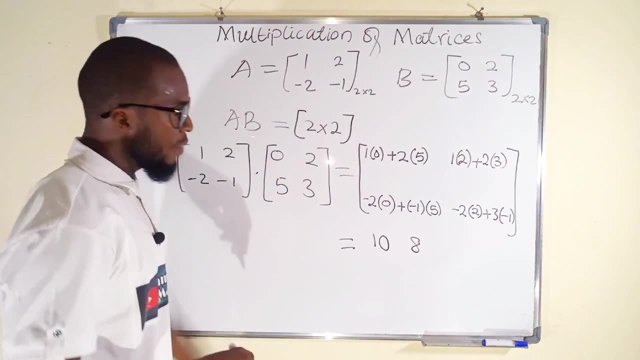 this is 2, because 1 times 2 is 2, this is 6,. 2 times 3 is 6, 6 plus 2 is 8, so we have 8 here coming down. we have: this is 0 and this is negative 5, negative 5 plus 0 is negative 5. 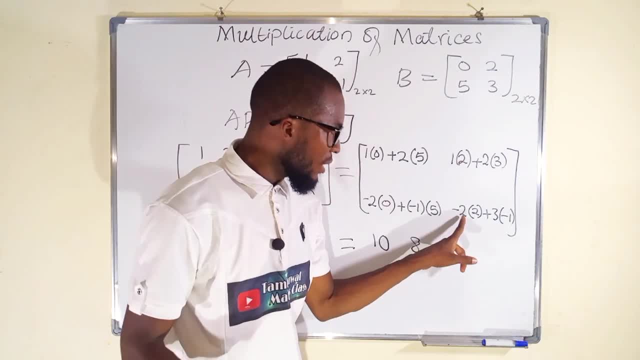 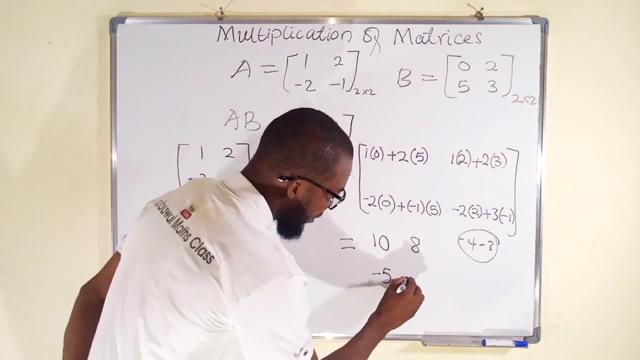 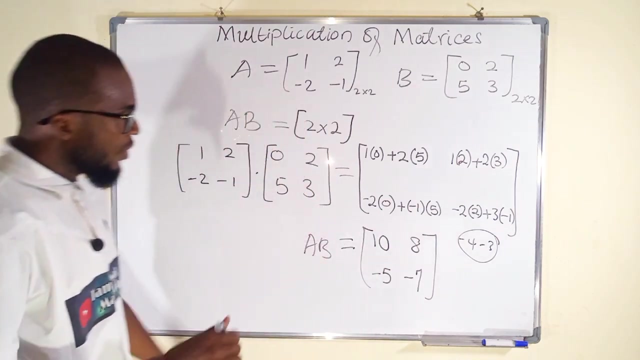 so we have negative 5 here. moving on here, this is negative 4, we have negative 4 and this is negative 3, all together, we have negative 7. this is negative 7, and remember, this is AB. you can see that after multiplying. 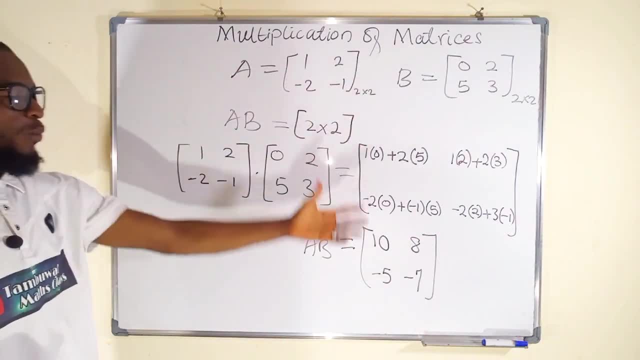 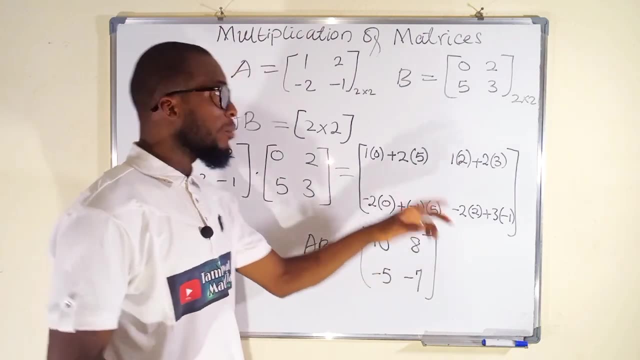 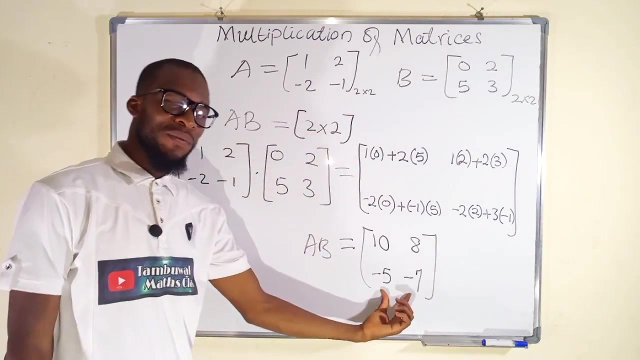 these two matrices together, we obtain another 2 by 2 matrix, because I told you you can know the order of the result by considering the number of rows here and number of columns here, which is 2 by 2, so we obtain another matrix, 2 by 2. 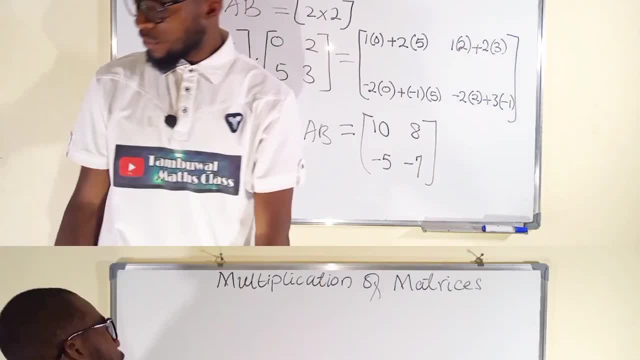 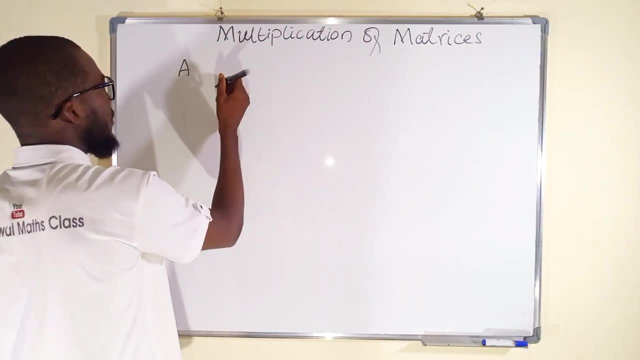 so we obtain another matrix 2 by 2. so we obtain another matrix 2 by 2. let's just take the last one. suppose we have a matrix A as 2, 1, 0,, 3,, 0,, 5. 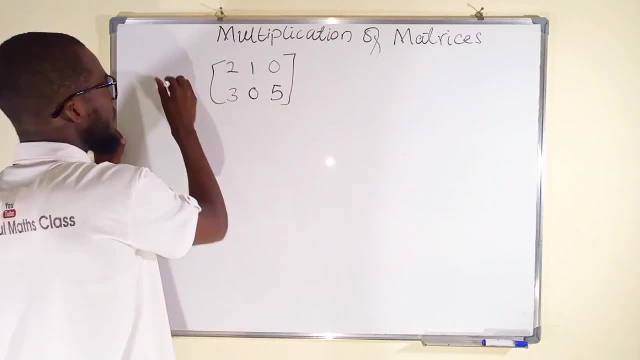 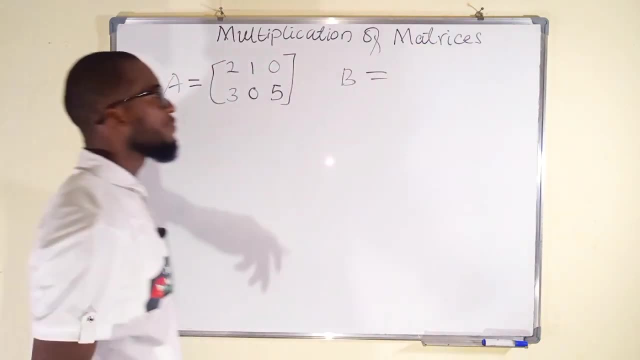 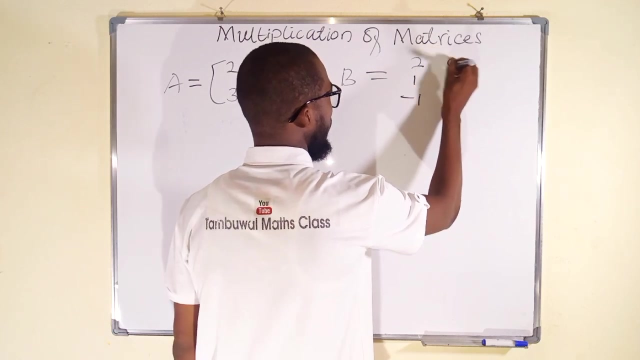 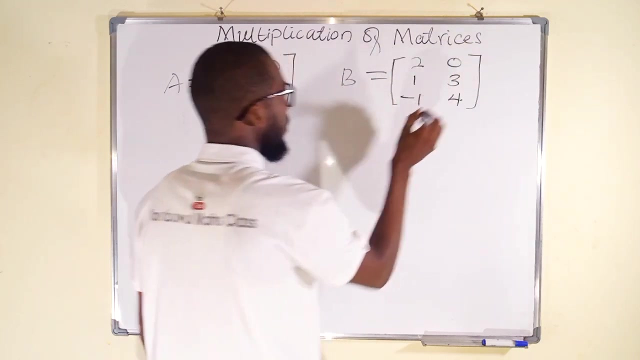 suppose this is matrix A and we have another matrix B as 2, 1, minus 1, and we have another matrix B as 2, 1,, 0,, 3, and 4, and we want to find A multiplied by B. 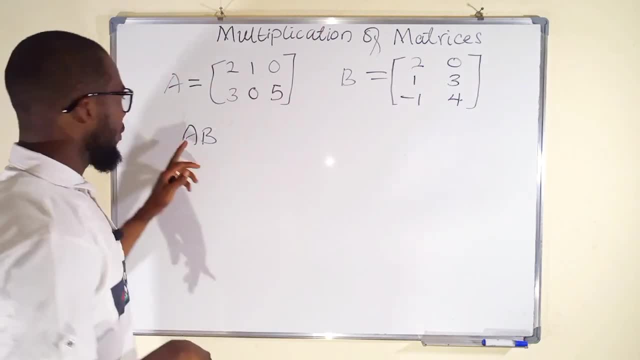 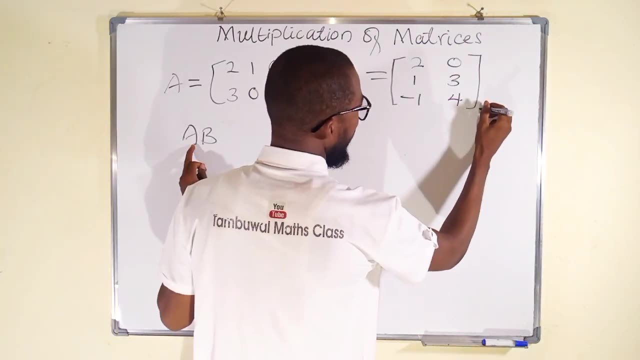 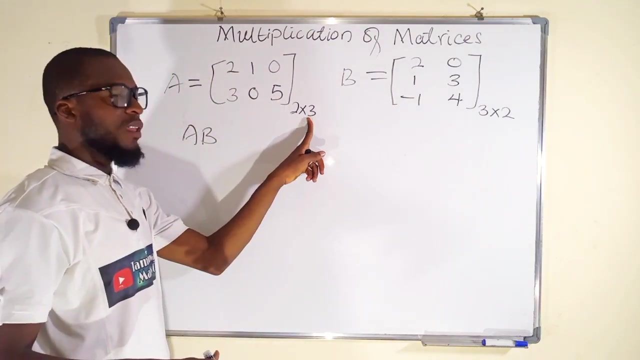 first thing we check for the compatibility. the number of columns: here you can see this is 2 by 3 matrix. this is 3 by 2 matrix. and the number of columns: here you can see they are 3. number of rows: here they are 3, so we can multiply them together. 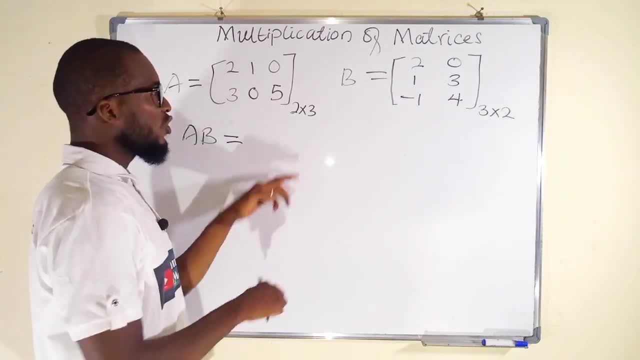 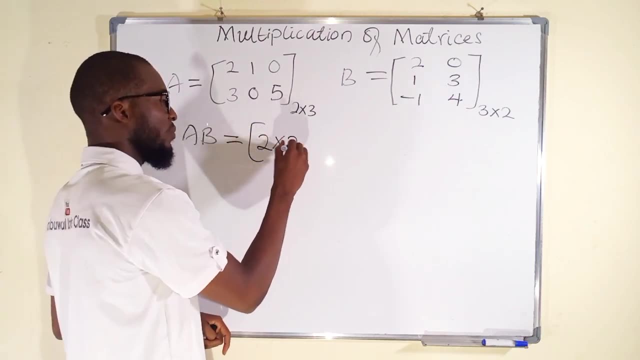 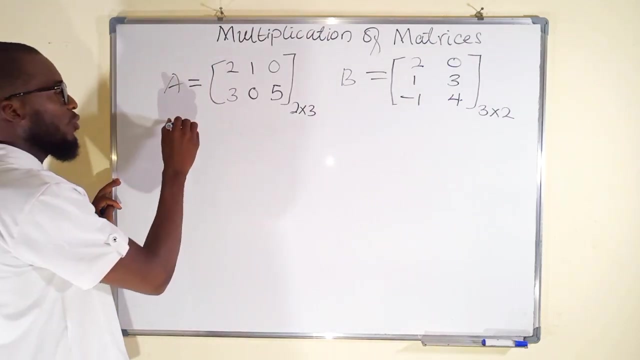 and the for the result. the order is going to be of: row here, column here: 2 by 2, we are going to obtain a matrix of 2 by 2. so now let us get started. we want to find AB, which is going to be for A. 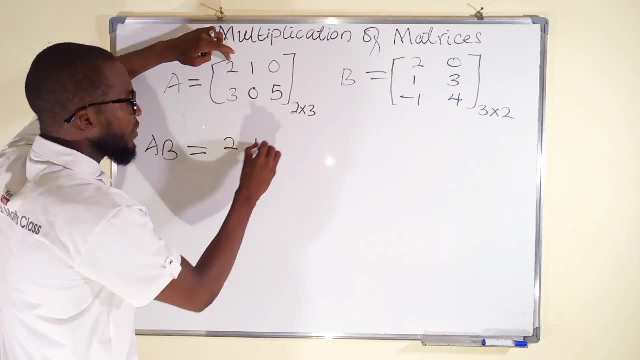 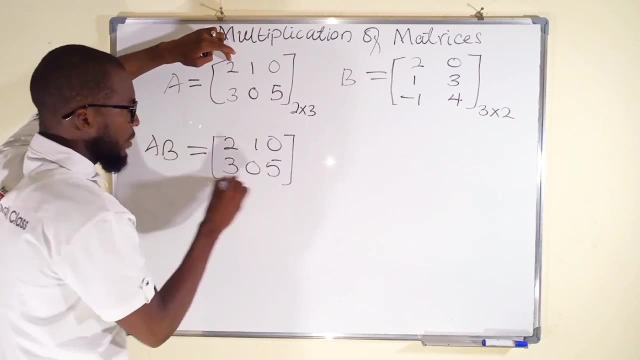 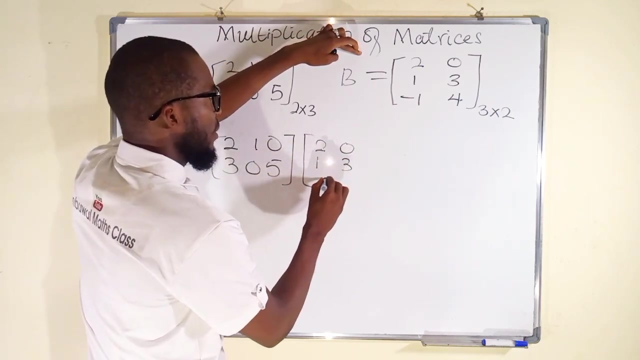 we want to find AB, which is going to be for A. For A, we have 2,, 1,, 0,, 3,, 0,, 5.. And for the second matrix, we have 2,, 0,, 1,, 3,, negative 1, and 4.. 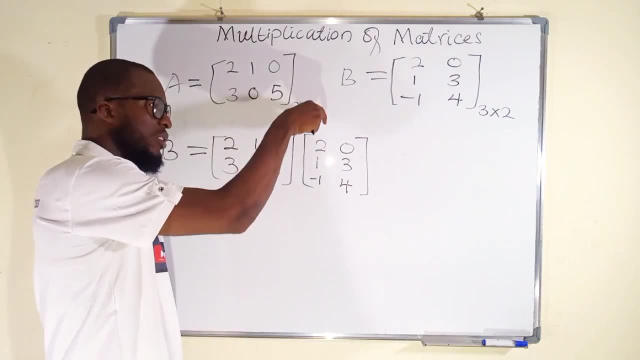 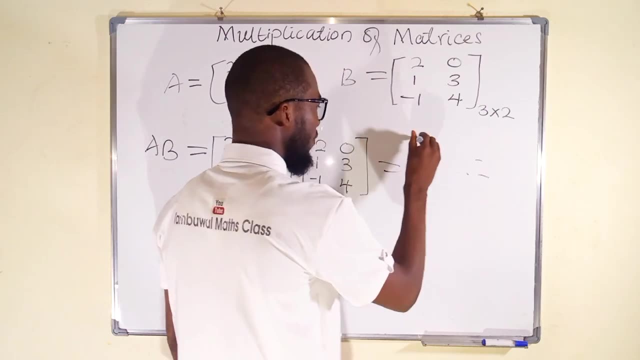 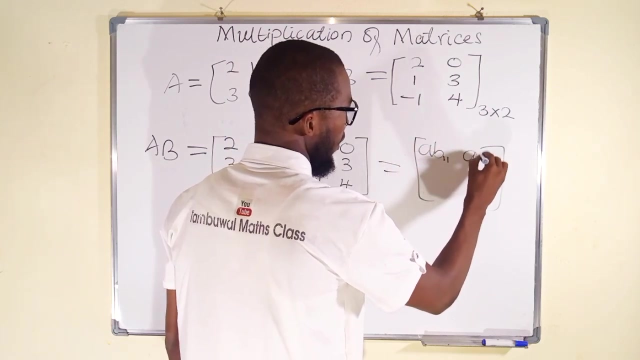 As always, we take the first row here. We multiply by the first column. Remember this is going to be a 2 by 2 matrix, So it is going to be of the form AB11,, AB12,, AB21,, AB22.. 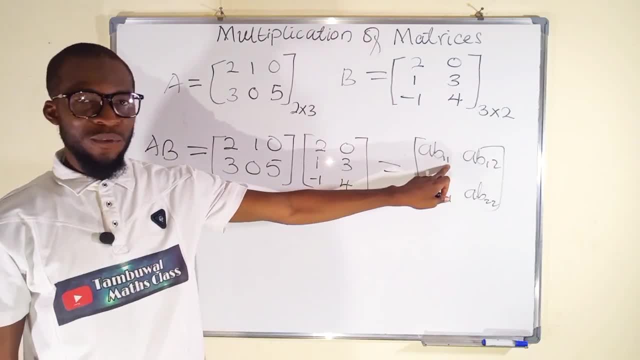 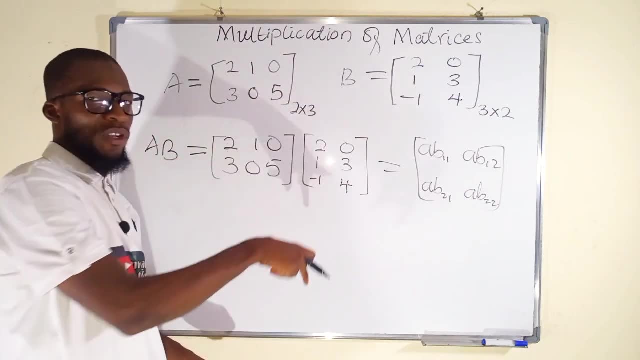 So to find this element at 1, 1 position, we're going to take the first row here from the first matrix and multiply by the first column from the second matrix. So let's begin. We say, okay, let me do it here. 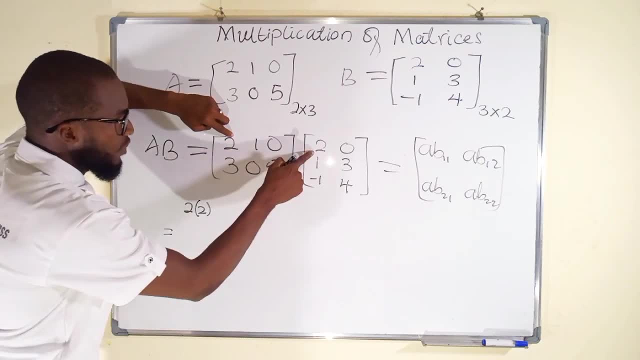 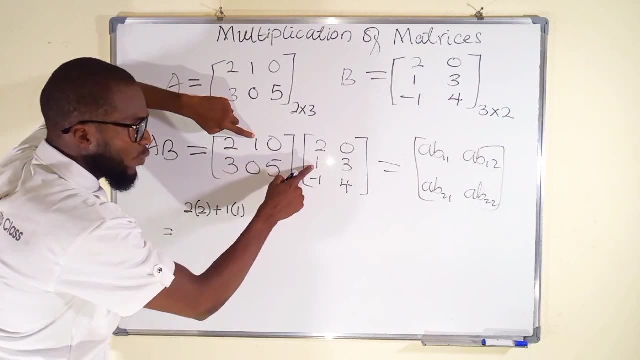 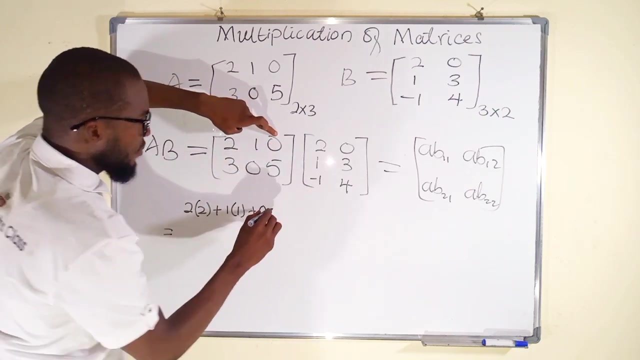 2 multiplied by 2. This, 2 and this 2.. Then you take this second element here, Plus 1 multiplied by 1. This 1 and this 1. They must correspond. And finally, this and this, We have plus 0 times negative 1.. 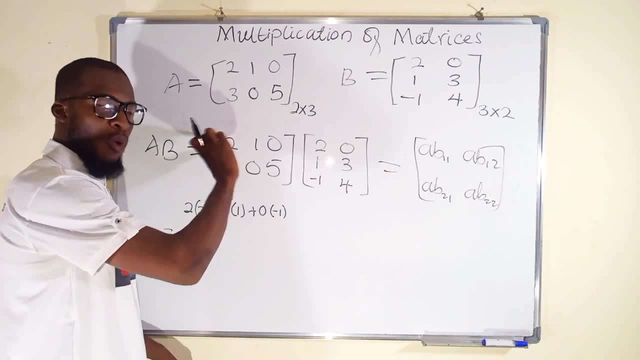 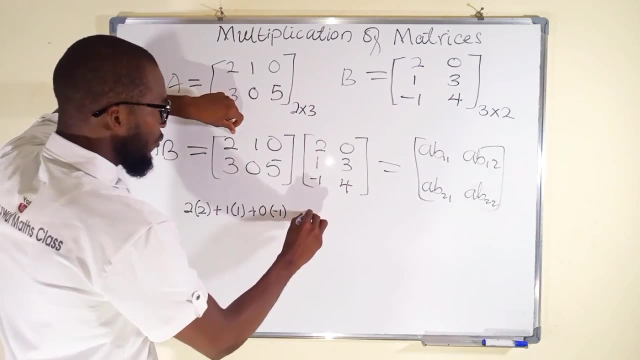 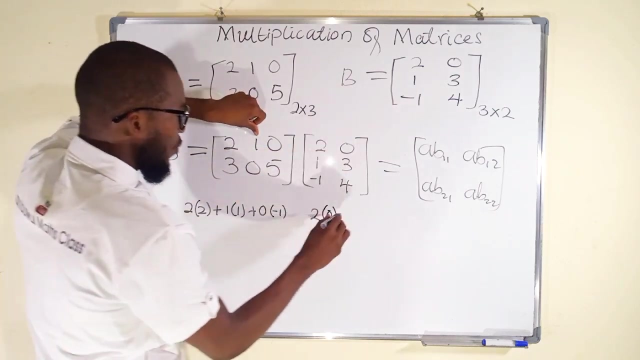 Then you give a space. Take the same row, Multiply by the second column to obtain 1, 2 position. We have 2 multiplied by 0.. This row and this column second, We take 1.. You always add. You multiply by 3.. 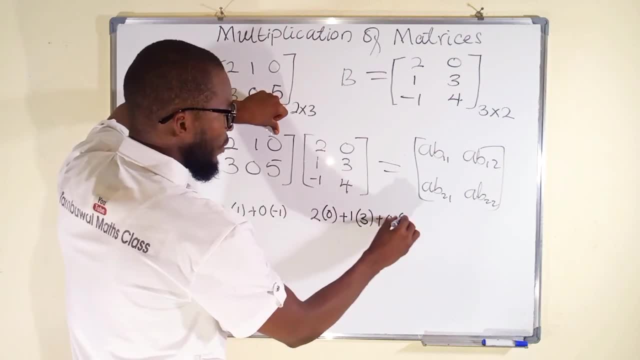 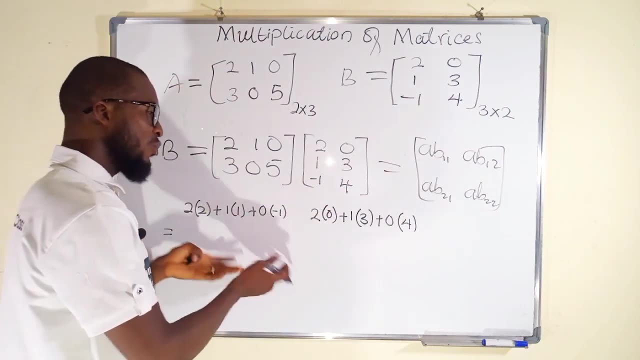 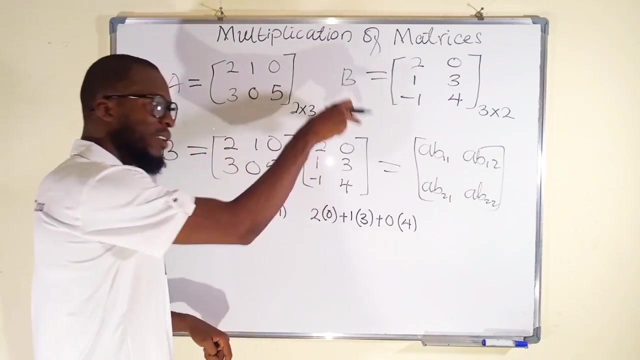 Then, lastly, you take 0.. You multiply by 4.. Remember, it is 2 by 2.. We have already obtained our two upper elements. Then, for this element, you take the second row. You use the second row to multiply these two columns. 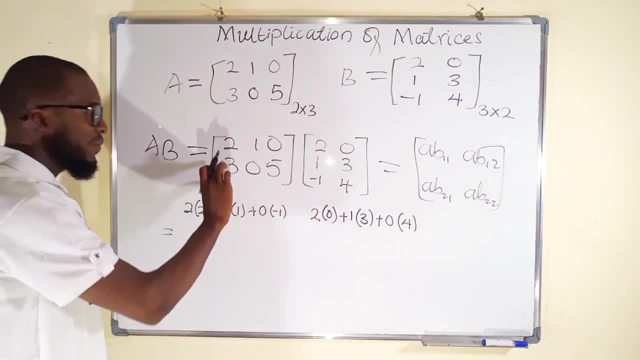 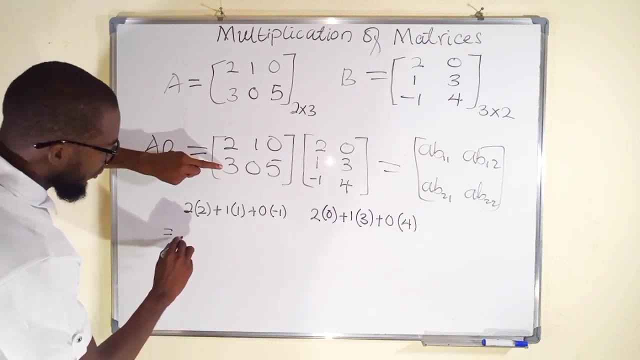 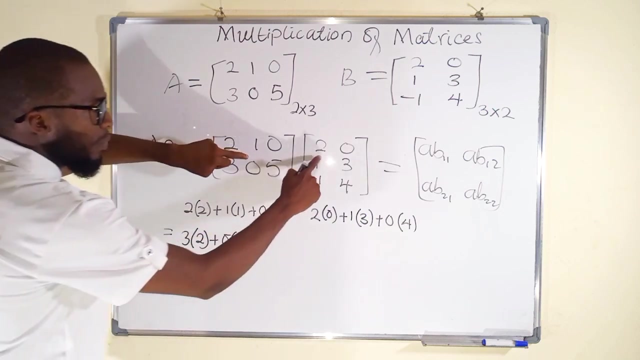 We have used the first row to multiply these two columns. Now it's left for us to take the second row, Multiply by the two columns. For this we have 3 multiplied by 2.. We add, We take 0.. We multiply by 1.. 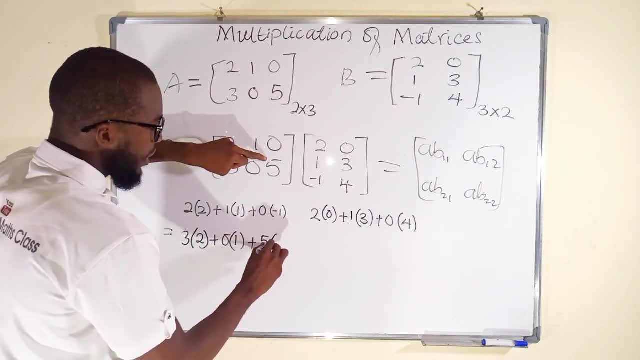 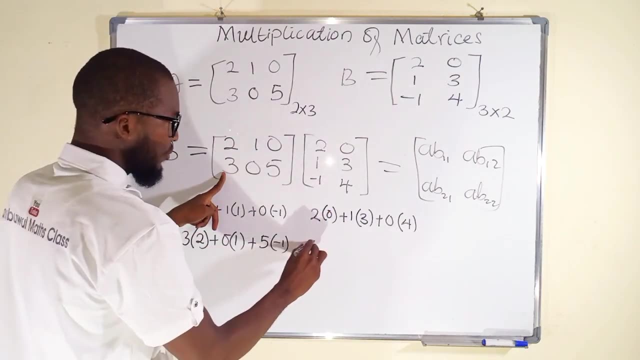 We add, Finally, we take 5.. We multiply by negative 1.. We give a space, We take the same row and multiply by the second column: 3 multiplied by 0. This is 0.. Plus 0 multiplied by 3.. 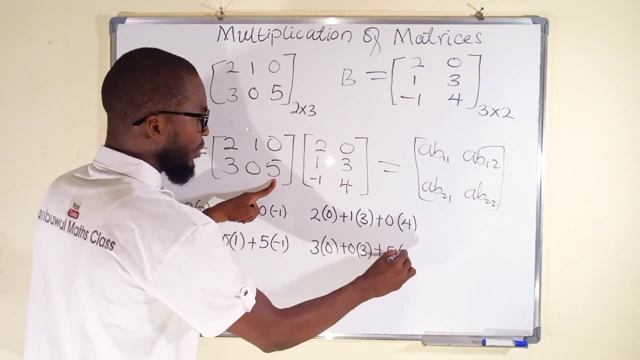 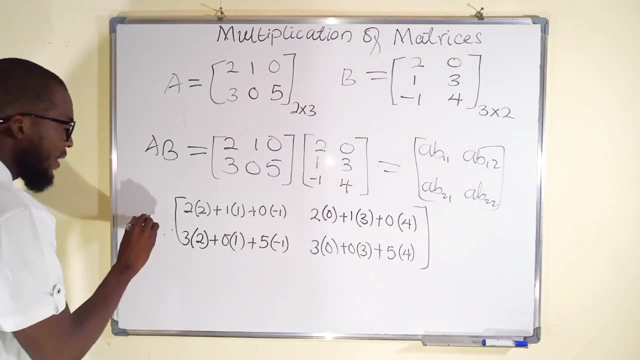 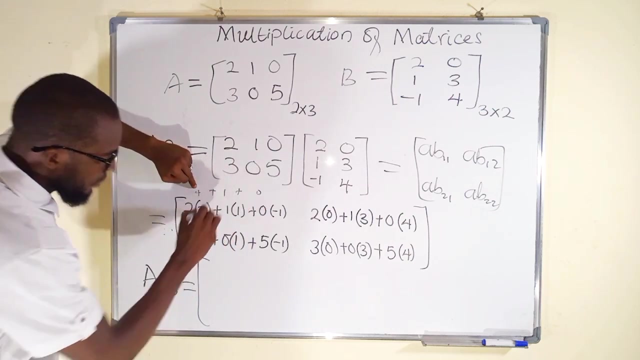 Lastly, we have 5 multiplied by 4. And we simplify to obtain our final answer. Finally, a b equals. let's do the work in here: This is 4,, this is 1,, this is 0,. 4 plus 1 is 5, plus 0 is 5, so we have 5 here. 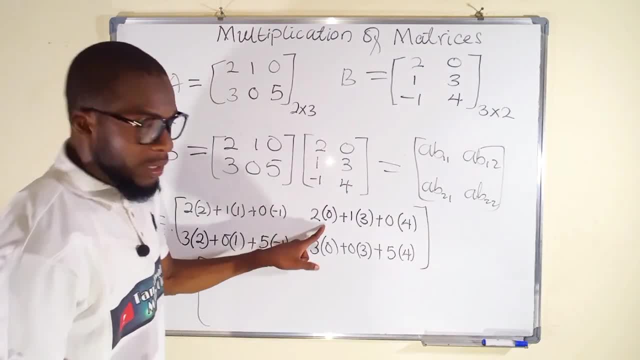 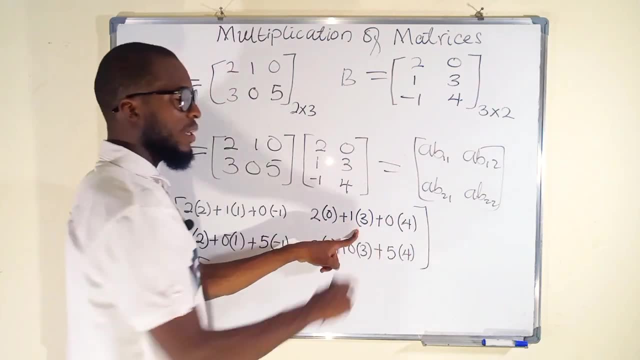 This is 0.. 2 multiplied by 2.. 2 multiplied by 0.. This is also 0.. 0 multiplied by 4.. This is the only element we have. 1 multiplied by 3 is 3.. Moving down here, this is 0.. 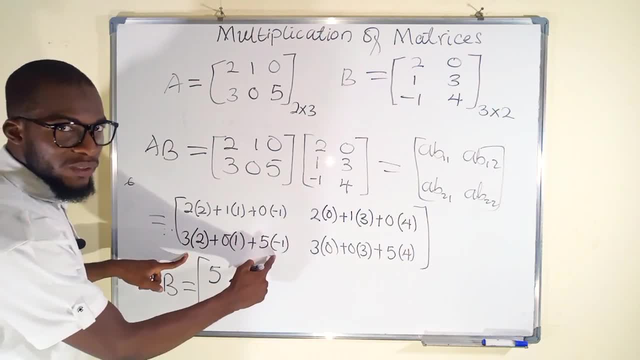 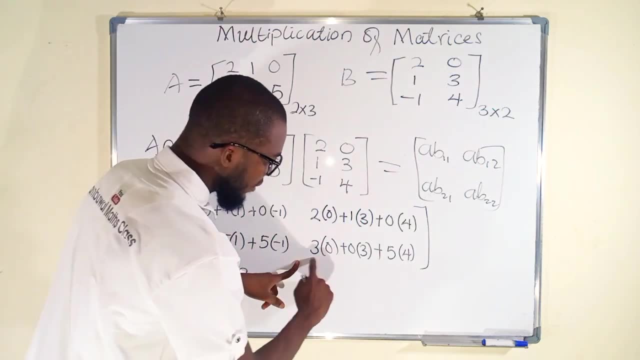 This is 6, so we have 6 here. 5 multiplied by negative, 1 is negative 5.. 6 multiplied by 5 is 1, so we have 1 here. Moving on here, this is 0, 0..